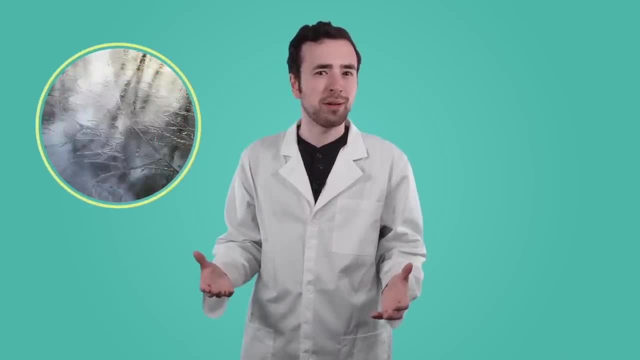 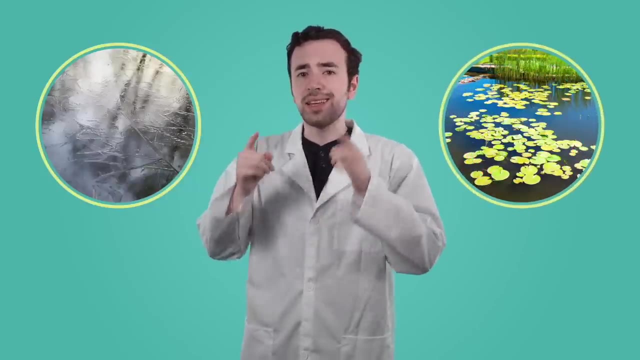 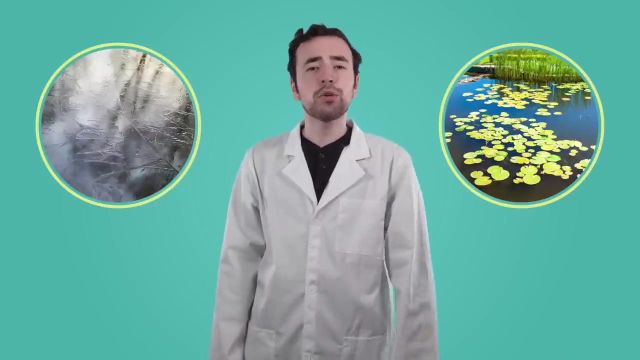 why can't we go swimming in a frozen pond? No, I'm serious, Think about it. Ice and water are all made up the same stuff, right? So why is it easy to move through water, but ice is all hard and tough? Well, to answer that question, we're going to need to learn more about the states. 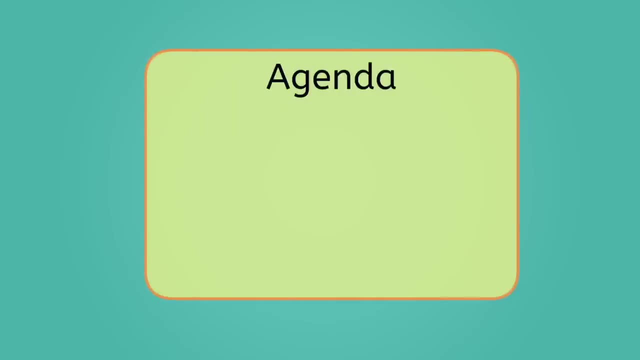 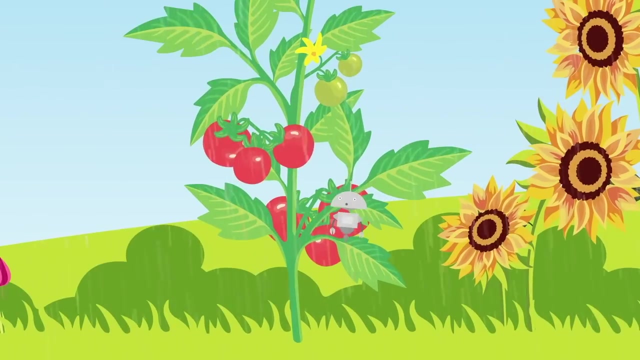 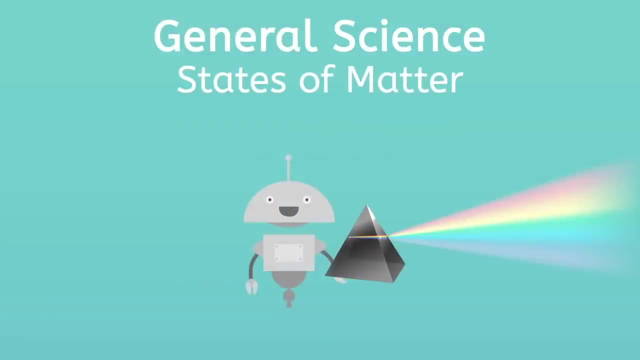 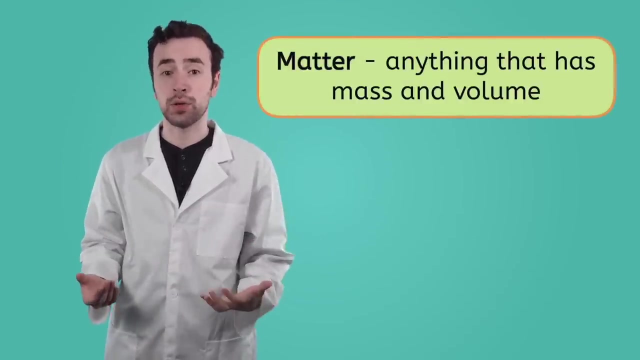 of matter. By the end of today's lesson, you will be able to identify the four states of matter and describe their properties. Let's get into it. In our last lesson we learned that matter is anything that has mass and volume. This means 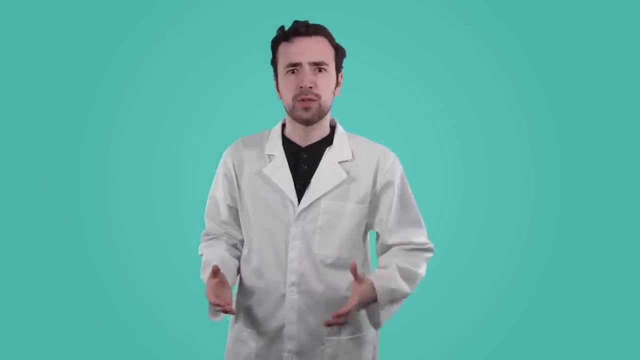 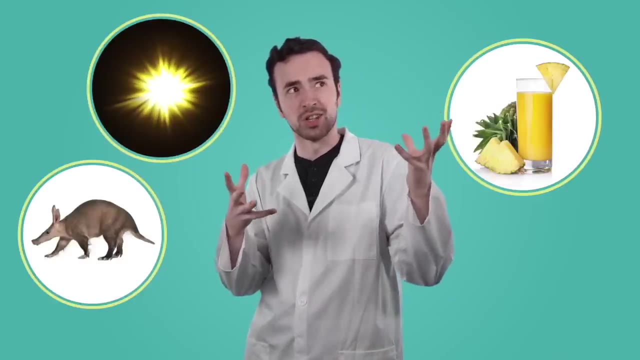 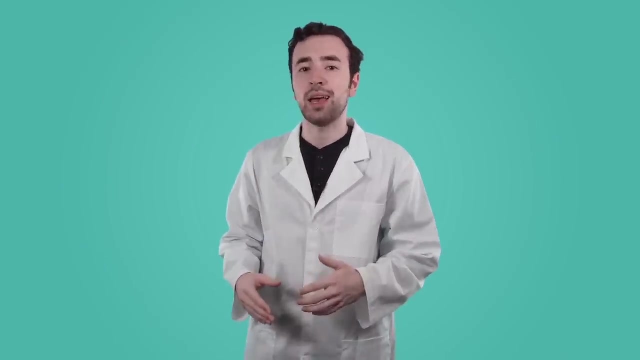 that wildly different things can all be matter, from an aardvark to pineapple juice, to the hydrogen and helium gases that form the stars of our universe. So, as you can see, matter comes in all sorts of shapes and sizes and states. What is a state? 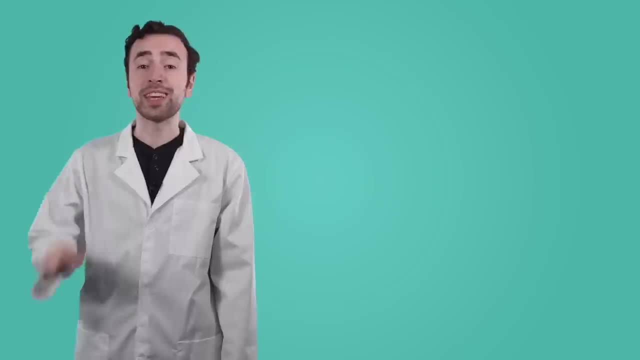 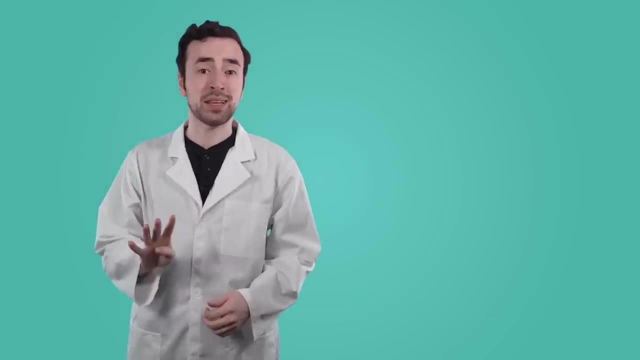 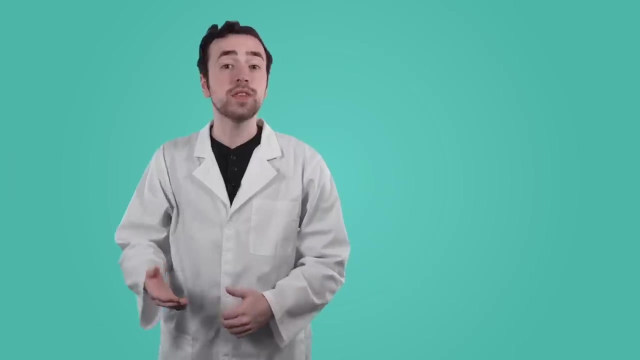 Well, state is one of those words with more than one definition, but in this case it means the form that matter is in. Matter comes in four different states: Solid, liquid, gas and plasma. Each of these states have certain properties that will tell us how the 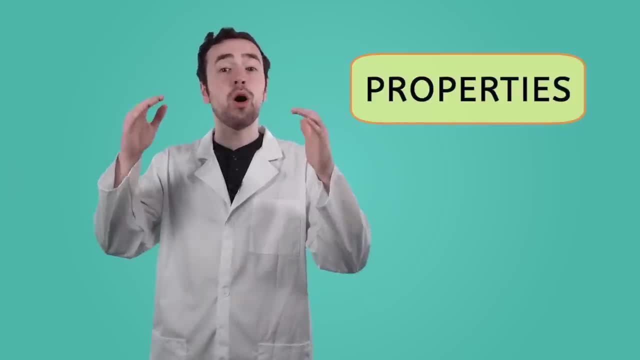 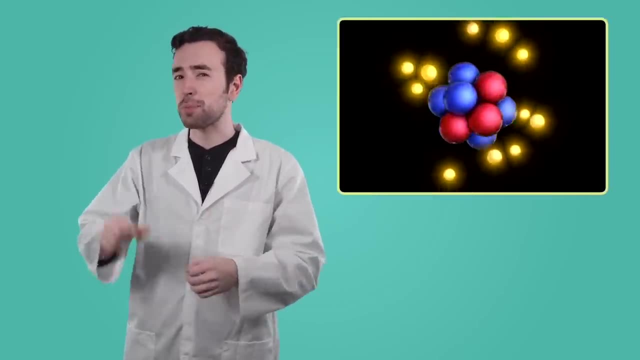 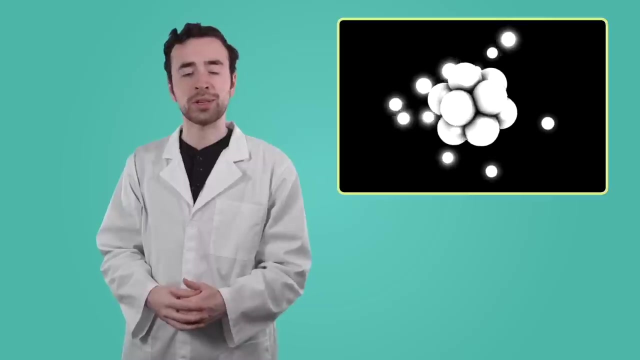 matter will behave. These properties come from all the way down at the atomic level. Remember in the last lesson when we learned that all matter was made up of teeny, tiny atoms. Well, it's how these atoms are arranged that will tell us what state the matter is in. 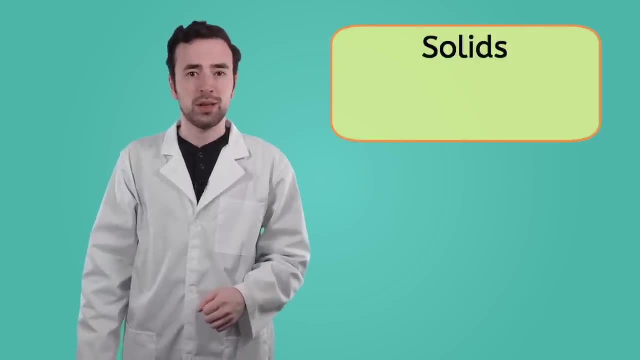 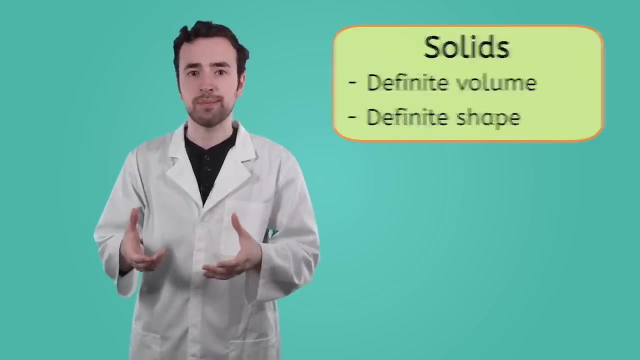 Let's take a look at solids first. A pencil, a baseball and the device you're currently using to watch this video are all great examples of solids. Solids all have a definite or fixed volume and shape. Think about this way: This rock. 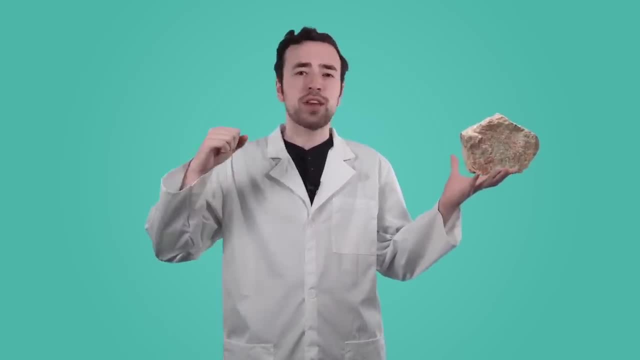 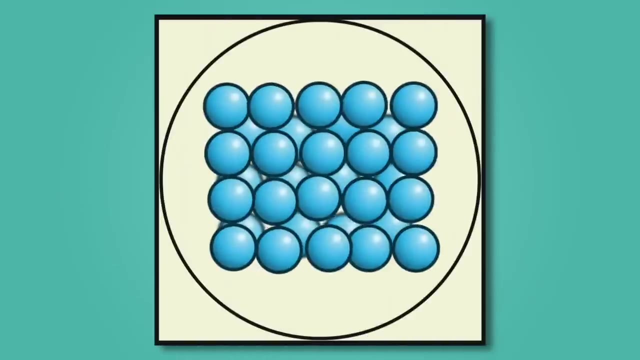 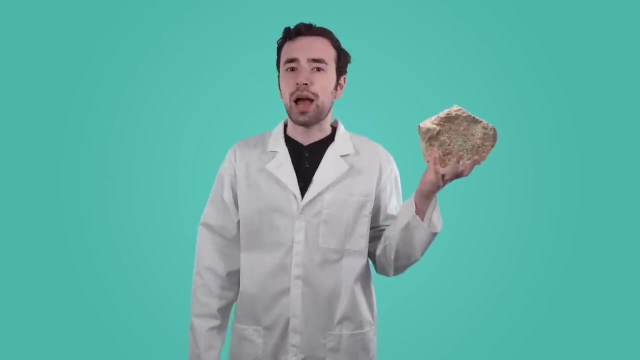 is a solid Right. Unless an outside force acts on it, it always keeps its same rocky size and same rocky shape. The reason for the rock's definite shape and volume is the arrangement of its atoms: atoms- A solid's atoms are packed extremely close together. Now let's learn how the atoms 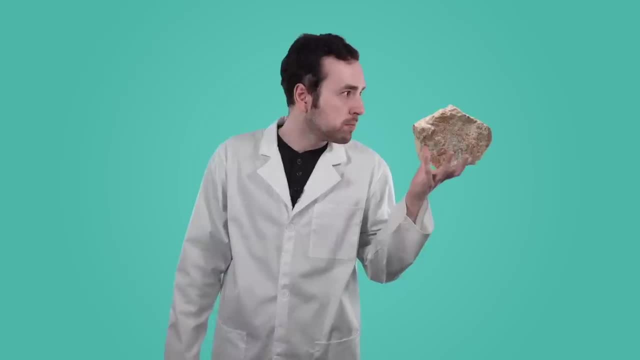 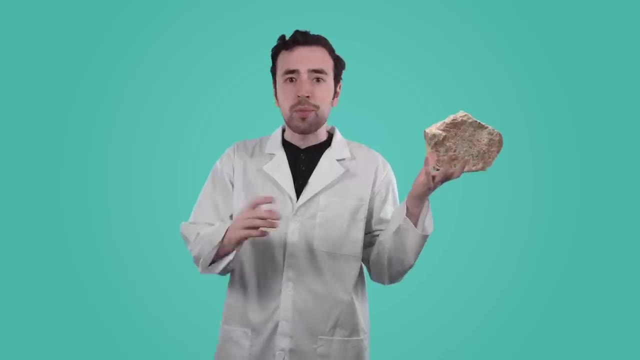 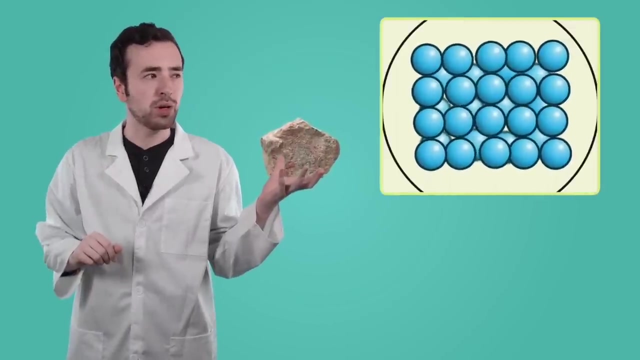 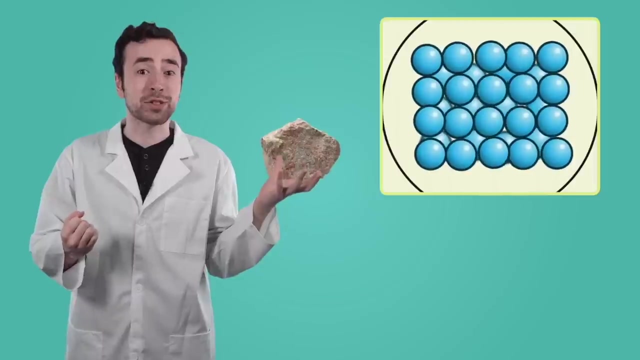 in a solid move by observing this rock Fascinating. Now you might think that solids don't really move much, and you'd be right. But once again, if we take a much closer look, you'll see that the atoms are actually moving. Now the atoms are really packed tightly together. 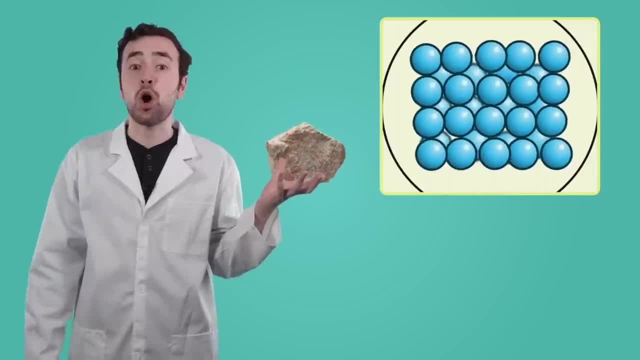 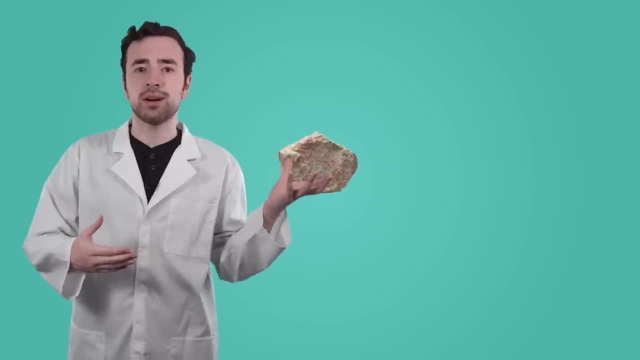 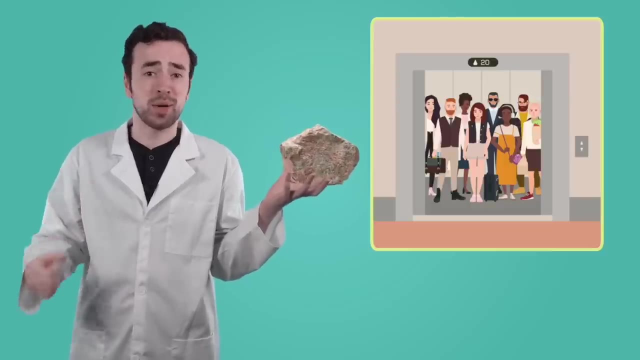 so they can't move much. but the atoms in a solid are all constantly vibrating Just a little bit. You can think of solids like a really tightly packed elevator. The people in the elevator are all cramped in there so they can't really move, but they're all. 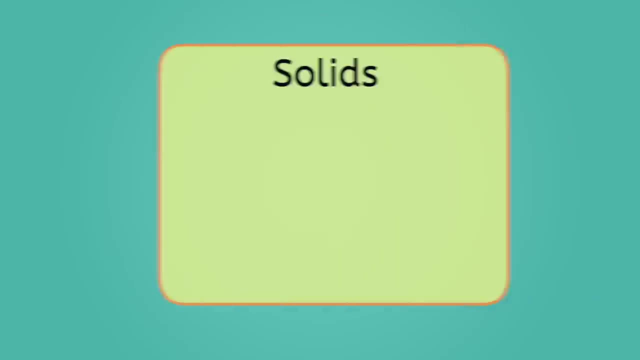 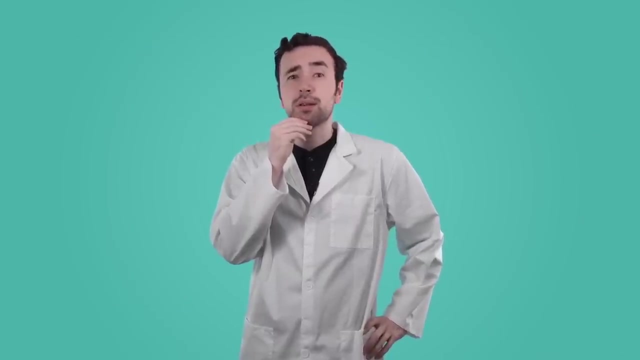 still kind of shuffling around just to get comfortable. So solids have a fixed shape, Shape and volume. Their atoms are packed very closely together and they're always vibrating. Hmm, What examples of matter in the solid state can I think of? Well, a donut is a solid. 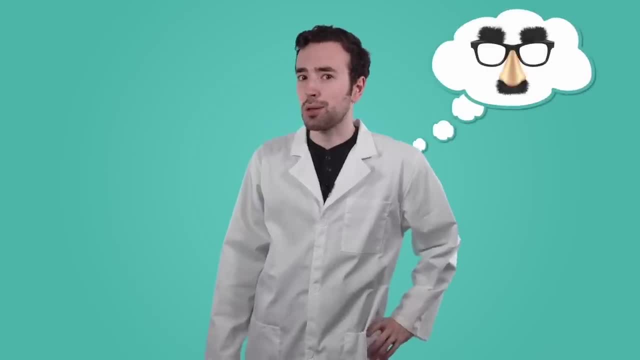 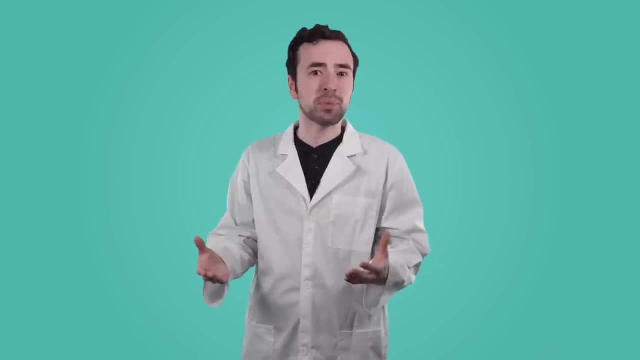 My pencil sharpener is a solid, And those really cool glasses that I got for the last lesson are also a solid. Why don't you pause the video here and jot down some of your own examples of the solids you can see around you in your guided notes? 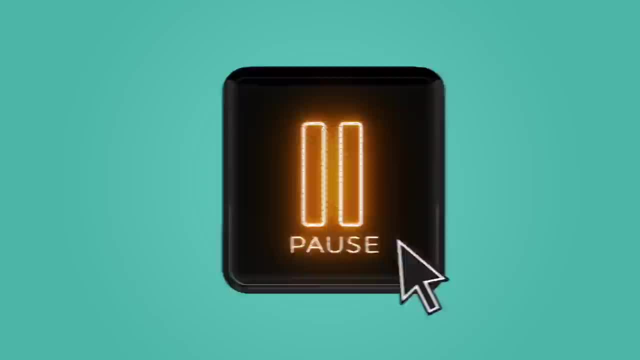 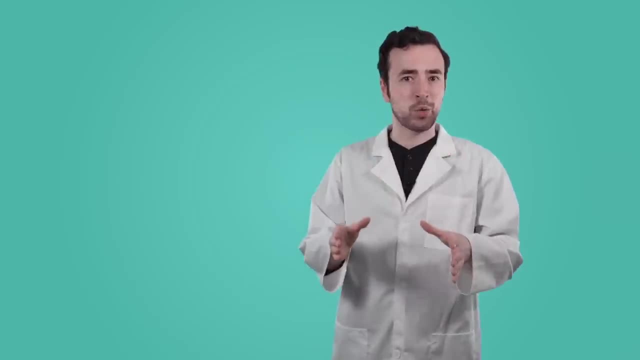 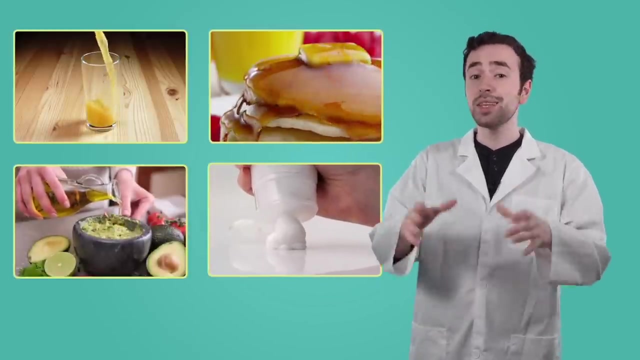 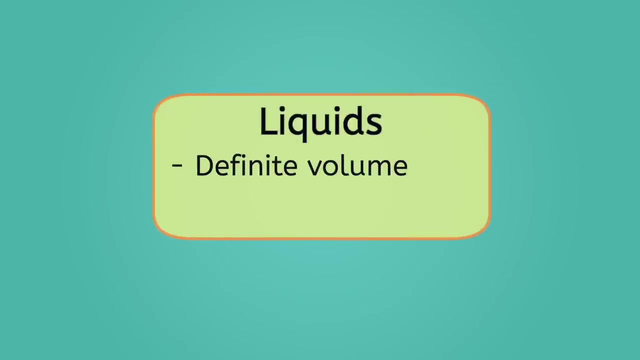 If you've had anything to drink today, then you have already come across our next state of matter. liquid Things like juice, syrup, oil and lotion are all typically in the liquid state when we use them. Liquids have a definite volume, so they always take up the same amount of space, However, 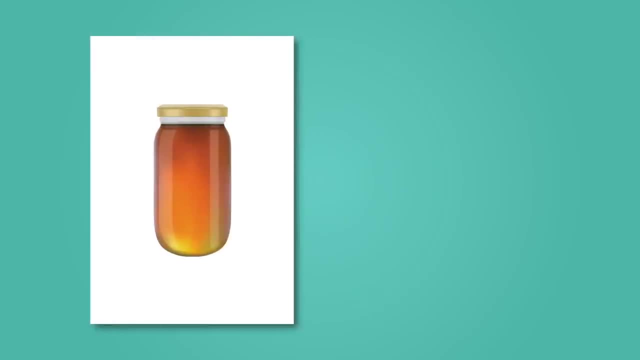 they don't have a fixed shape. If you pour a liquid into a cylindrical container, it will take the shape of a cylinder. Pour it into a bear-shaped container and it'll take the shape of a bear. Liquids take the shape of whatever container they're in. 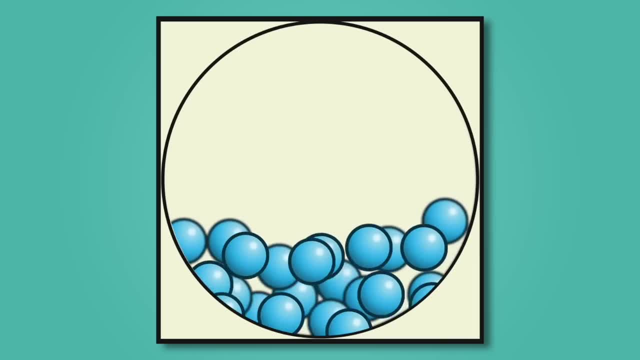 This is because the atoms in a liquid are more loosely packed than a solid. Because the atoms are more spread out, they can move faster and they're able to slide past each other. This is what allows a liquid to flow and be poured. 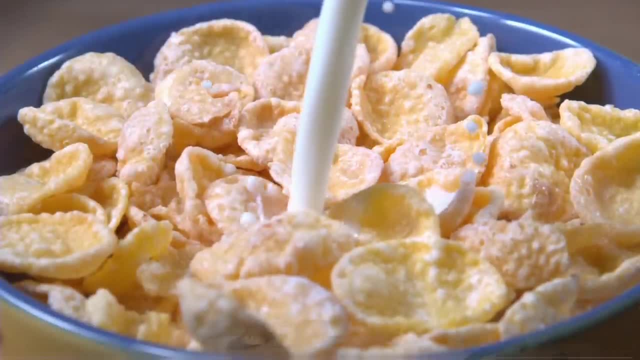 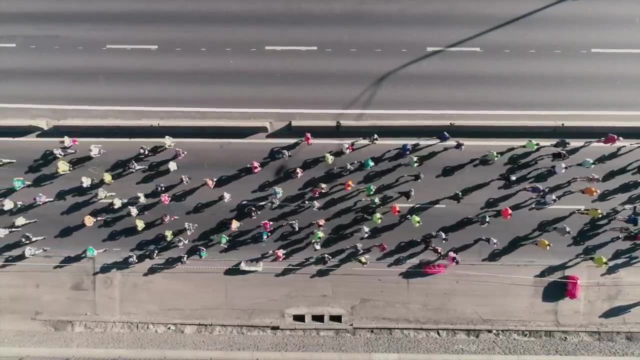 like when you pour milk into your cereal bowl. If solids are like a crowded elevator, then liquids are kind of like a race. It's still pretty crowded, but people are able to pass each other or fall behind And they are definitely moving faster than those people stuck in the elevator. 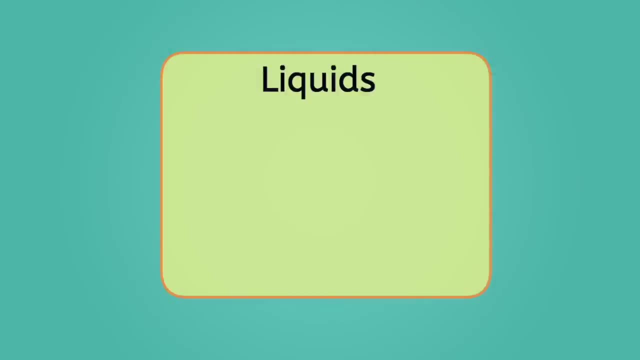 To recap matter, in the liquid state has a definite volume but no definite shape. Its atoms are more loosely packed, allowing them to move faster and slide past each other. Pause the video now and write down some examples of liquids in your guided notes. 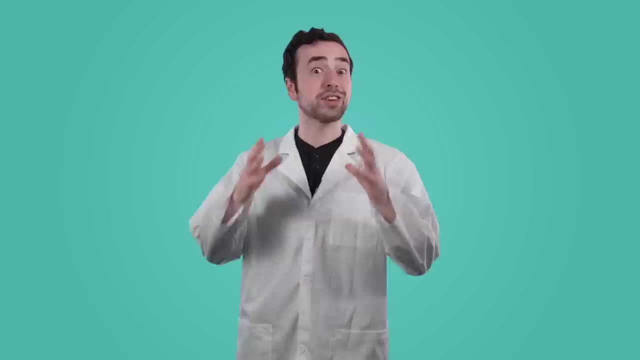 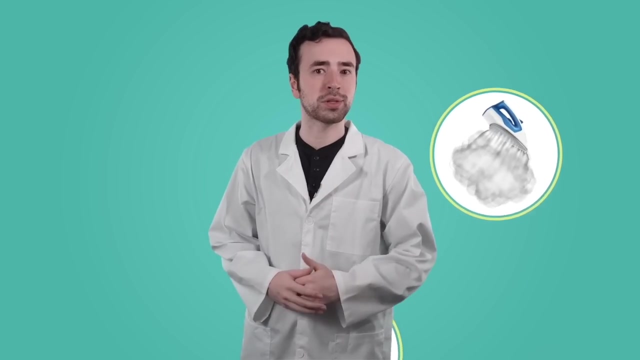 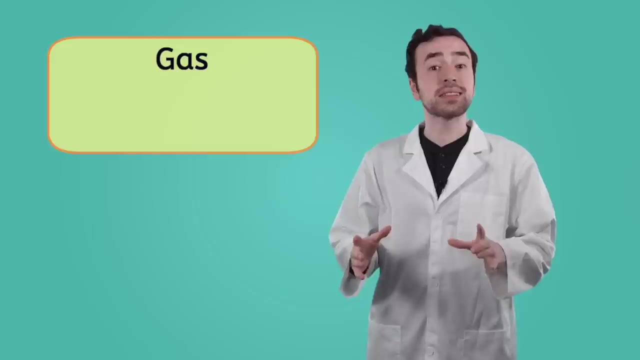 Our next state of matter is gas. Gas constantly surrounds us. We use helium gas to fill up balloons, steam gas to iron out the wrinkles in our clothes and, of course, we all rely on the oxygen gas in the atmosphere to breathe. Gases have no fixed volume or shape. 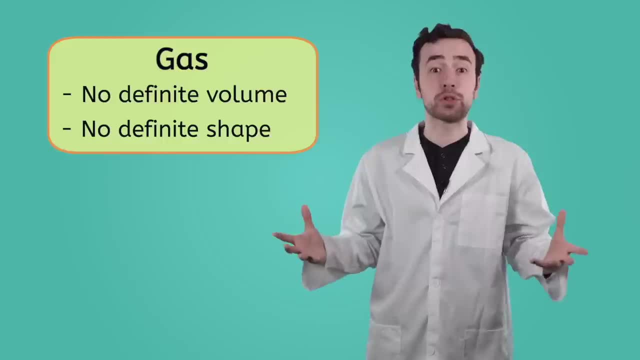 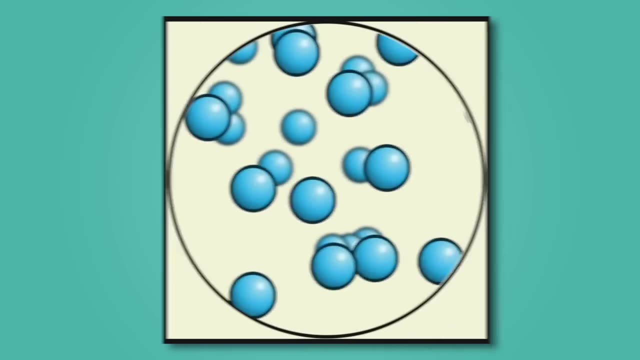 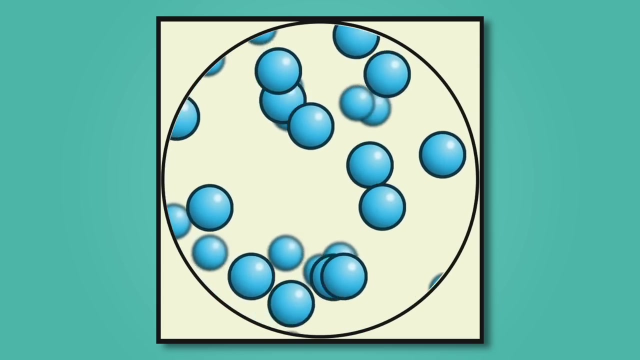 In fact, gases will expand into whatever space is available to them, whether that's a car's tires or an entire room. Gases behave this way because their atoms are very spread out. The atoms are moving super quickly past each other. They're kind of like kids running around a playground. 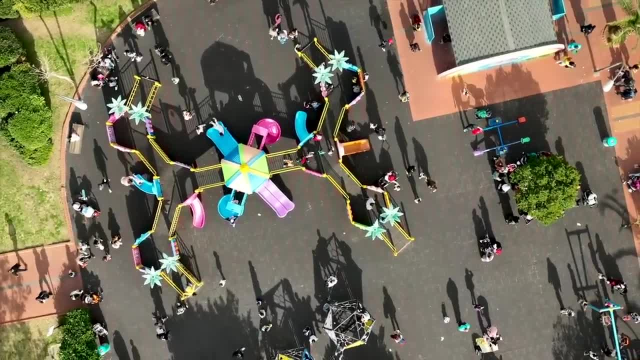 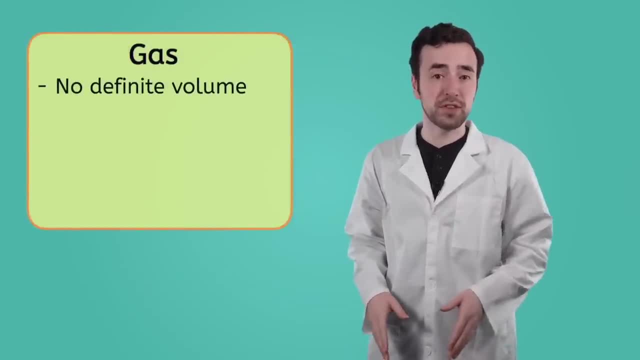 They are spread out, they're moving quickly in every direction and they might sometimes bump into each other, but that doesn't happen too often. So gas has no definite volume or shape. Its atoms are all spaced out and moving around really quickly. 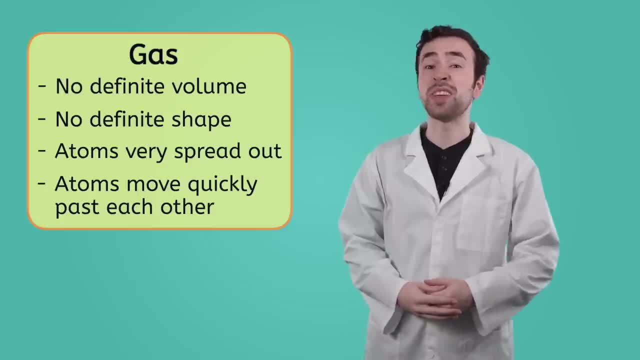 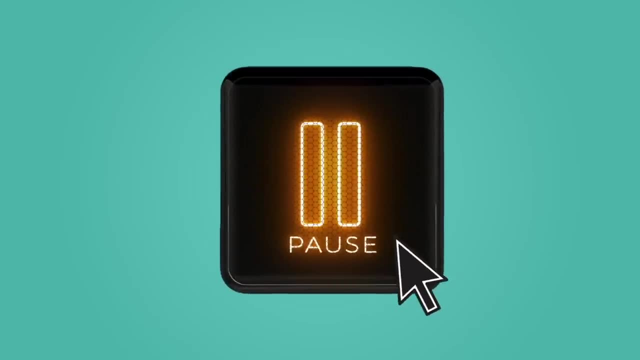 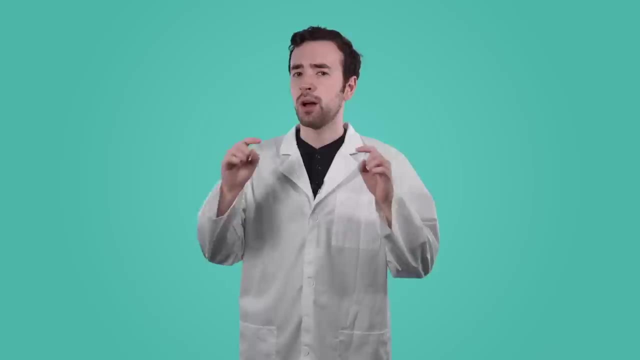 Pause the video now to come up with some of your own examples of matter in the gas state in your guided notes. Solids, liquids and gases account for most of the matter that we see here On Earth, however, about 99% of all matter in the universe.